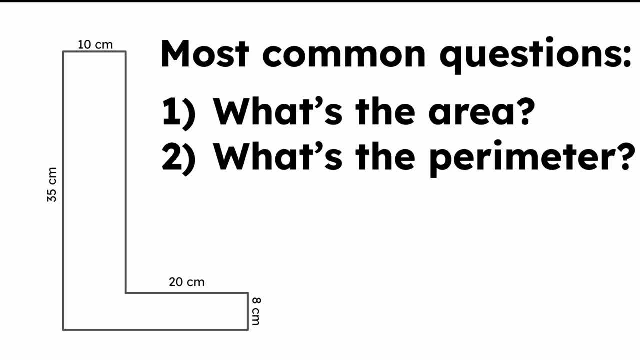 Well, it turns out, especially with the first one, the area, that there is a pretty simple way to do it. There's like a trick that you can use that will make this not confusing anymore. It'll make it pretty simple. And that trick ready. are you watching carefully? You see that. Do it again. All right, You just draw. 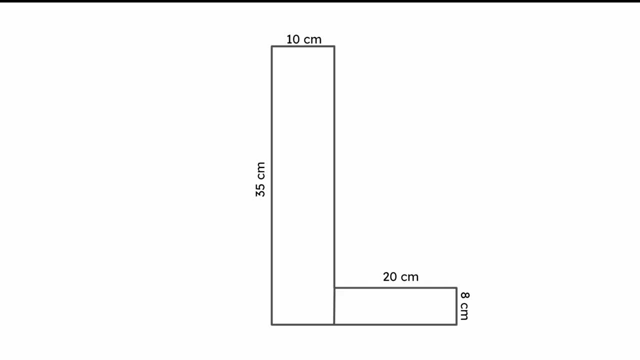 it a line. It's like magic. You take one shape and turn it into two shapes. Ding. That was another special effect right there. This is my videos are getting just more and more ambitious technically. I hope you're all appreciating that. Took me a long time. See that yellow, yellow and the wand- All right. 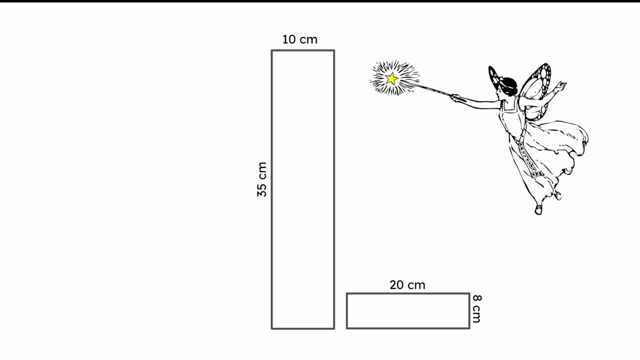 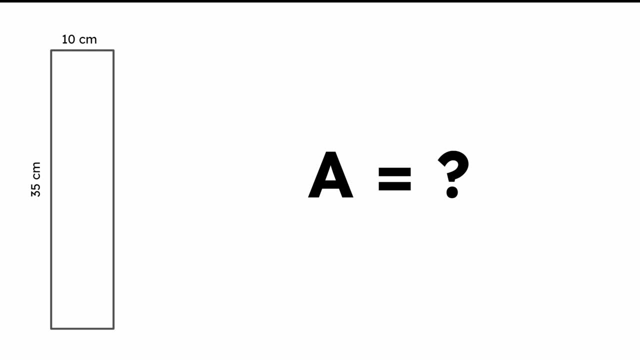 So what do you do if you have two uh rectangles? well, that's pretty simple. um, let's look at this first rectangle. here they're asking for area. maybe you know it off the top of your head. you don't have to, because the ged will give. 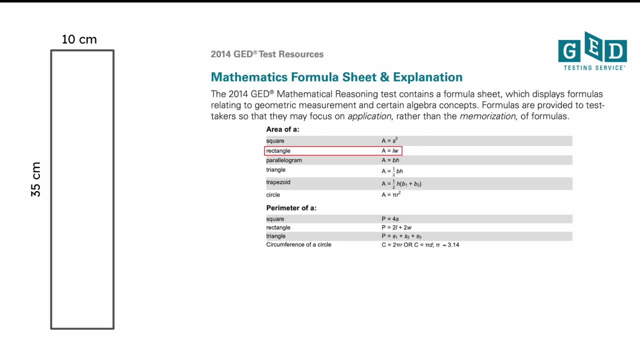 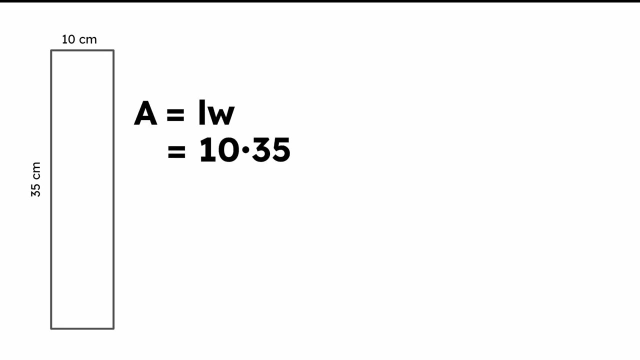 it to you on the formula sheet. it's right there: the area is equal to the length times the width. okay, well, the area is equal to the length times the width. i just said that. um well, what's the length? it's 35. what's the width? it's 10.. that's pretty simple. you just multiply them together. 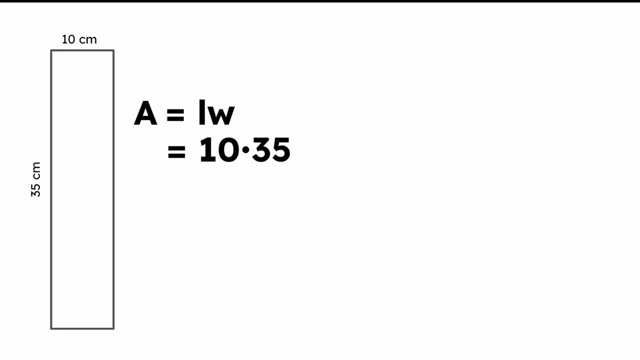 you can do this in your head if you want. if you are, if it's not one of the first five or six questions- the no calculator section- i would encourage you to use a calculator every time you do arithmetic, um in case you know. there's just no chance for a careless mistake, although 10 times. 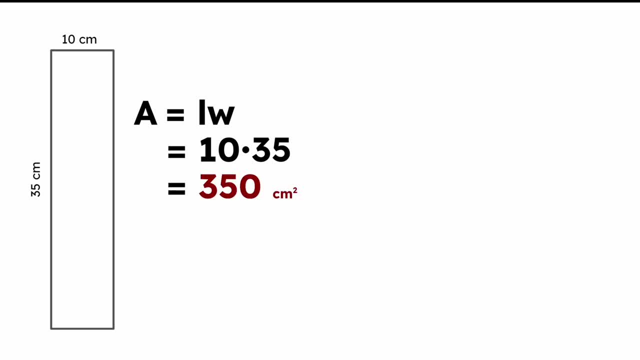 35 is about as easy as multiplication gets the other. the other one 8 times 20, same deal. probably do that in your head too. maybe i don't know. you don't have to. hopefully, if you have a calculator, 160.. so we have the two, uh. 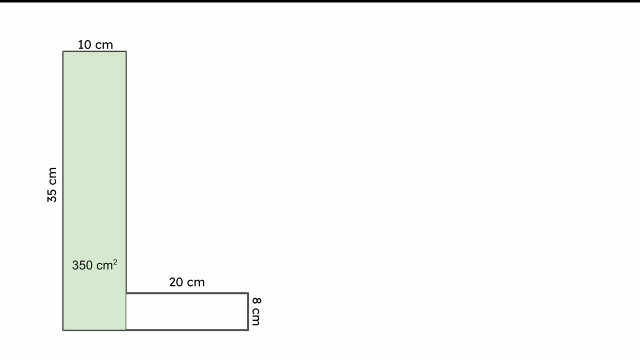 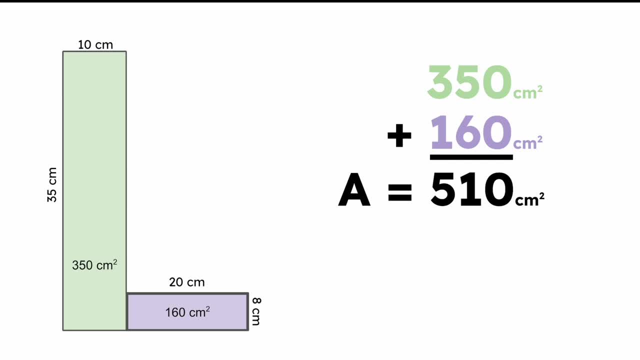 add them 510.. 350 plus 160.. What do you get? 510.. Nope, not a chant. All right, that's it for the area questions. They usually won't be much more challenging than that, Maybe a little more. 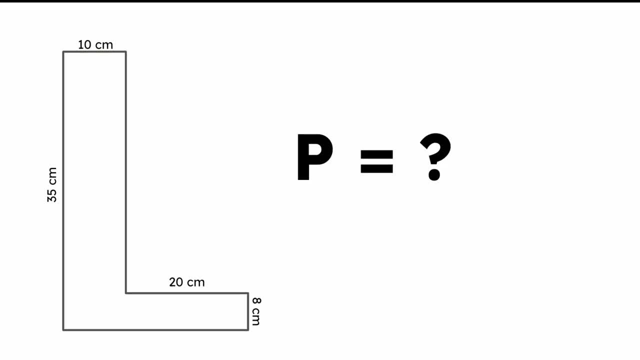 challenging. We'll get to the one at the end of this video is a little more challenging. All right, what about the perimeter? Perimeter, you may remember, is basically all the sides added up together. You can think of it as like if you were like a little dude walking around the 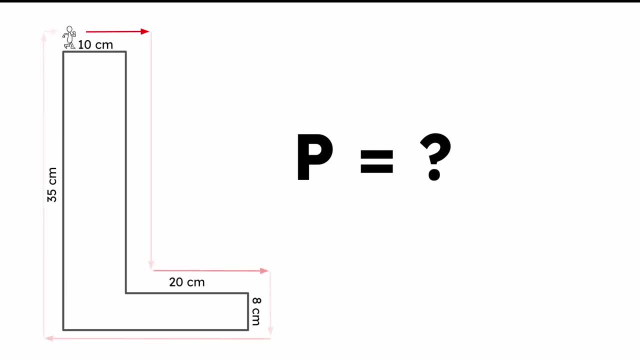 shape. what is the length you would have to walk to get from the very beginning to where you started? That's perimeter, More special effects. You all see this. Okay, the problem here is these two. are these two question marks? They don't tell you. 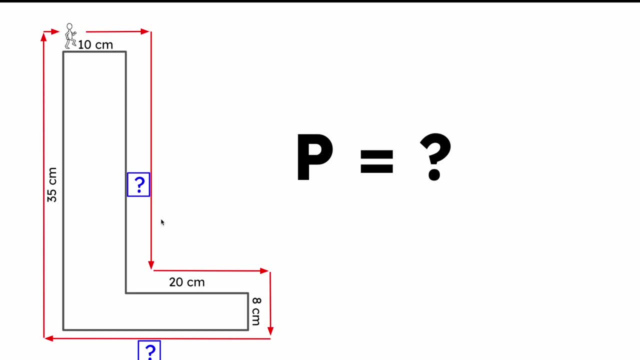 here we have. we know this is 10 centimeters and 20 and 8 and blah, blah, blah, but they don't tell you how long this is. How do you figure it out? Well, I'm here to help. Let's look at this bottom. 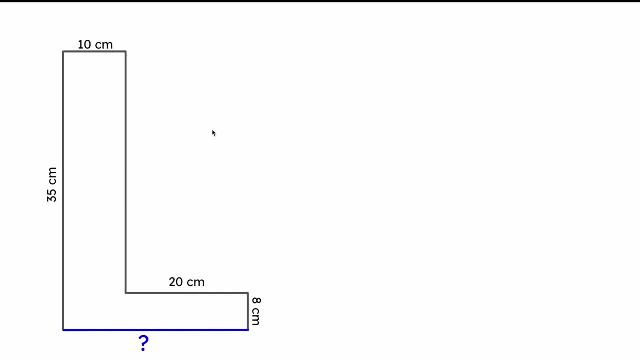 one first. We don't know what it is, They don't tell us. However, they do tell us other things that are kind of important. We know these two lengths, the 20 and the 10. And guess what? The 10,- you can just kind of like move down. It's kind of like the magical, weird trick I showed you with. 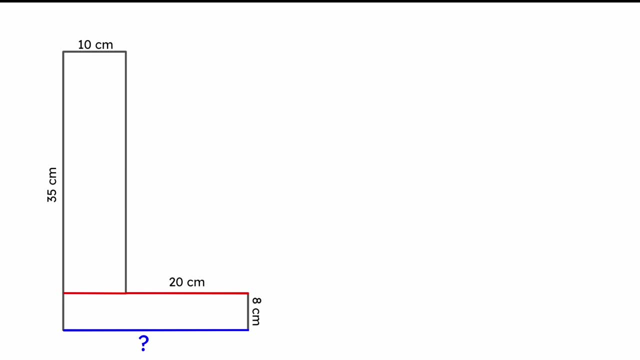 a thing: You just kind of like draw in a line and you know that line. that line is 10.. Well, if this is 20 and this is 10, the whole thing has to be: guess what guys? 30, 10 plus 20.. Now you know. 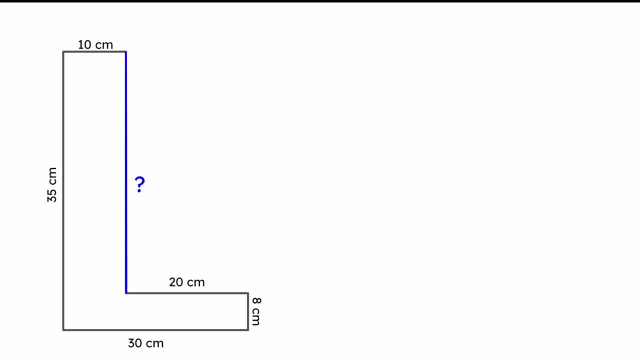 you know, the blue thing, Great One down, one to go. This one is sort of the same, except in reverse. We don't know this and we don't know the pieces of this we can add together. However, we do know. 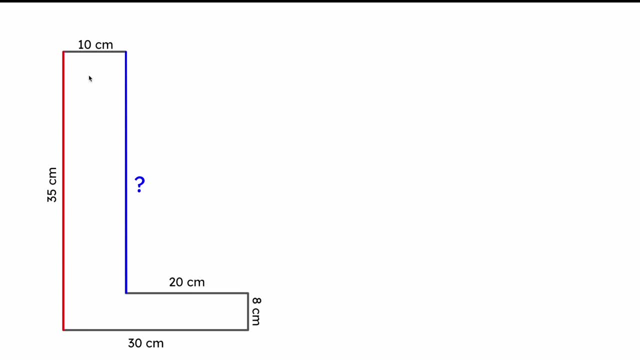 this is 35, from the very bottom of the shape to the top 35 centimeters. We also know that, whatever this is, if we just take it away, that's what's going to give us the blue line, right? This is missing from the blue line. Well, guess what? We know the blue. 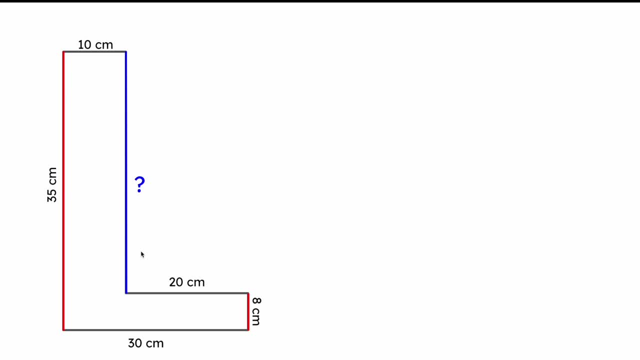 that little red piece. it's eight centimeters, So 35,. take away this eight centimeter length, That's going to be our blue line 27.. See, easy, And now we know all of the sides: 10,, 27,, 28,. 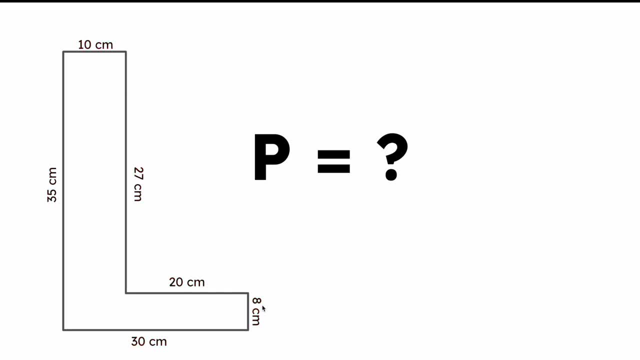 30, and 35. We just add them together. What do you get? I'm tempted to do another chant, but I learned my lesson the first time, Did I? I guess we'll find out. Keep watching, We'll see if I learned my. 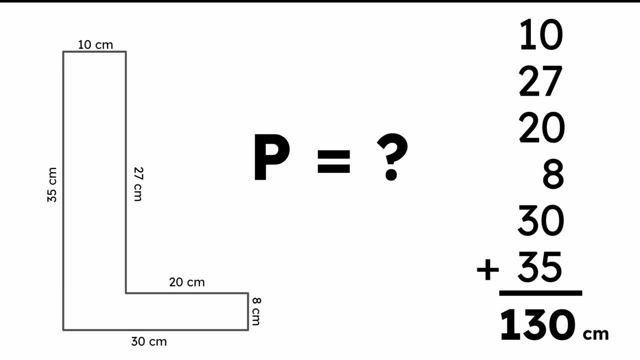 lesson. That's another thing right there. I would use a calculator for, if I had access to it, 130.. There we have the area, we have the perimeter. we figured it all out ourselves. Congratulations to us. Let's take a look at a GED style question. This shape is a little different. 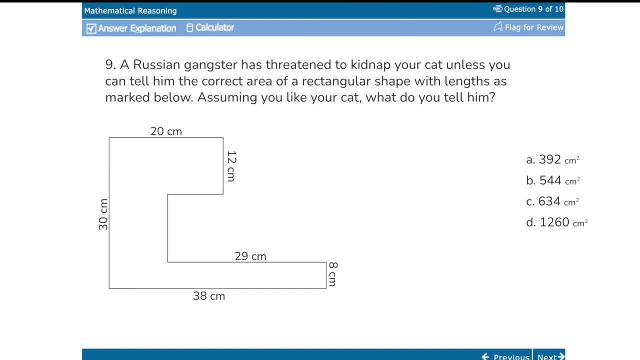 It's a little more complicated. It looks like, I don't know, a C got punched in its face, maybe, or it looks like a cartoon character trying to flex a bicep, a really kind of like weak bicep right there. I don't know if you can see that. 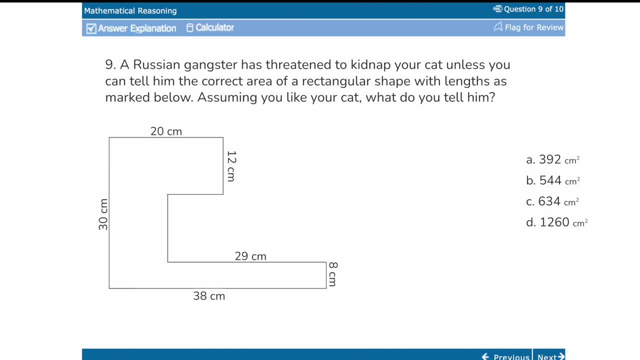 Got to go to the gym, bro, Anyway, All right. Again, we see we have a bunch of information and we are lacking some information. There are some sides we don't know And let's see what it's got. Let's see what's in here. This says: Okay, it's a Russian gangster, who is a Russian gangster? 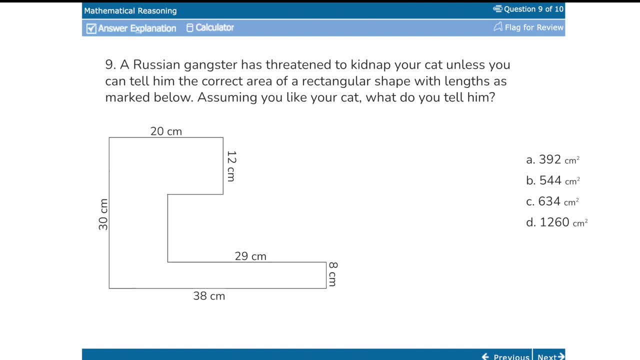 has threatened to kidnap your cat unless you can tell him the correct area of a rectangular shape with length as marked below. Assuming you like your cat, what do you tell him? All right, Well, what's that? one weird trick. I don't know what the area is going to. asking for area. I don't know. 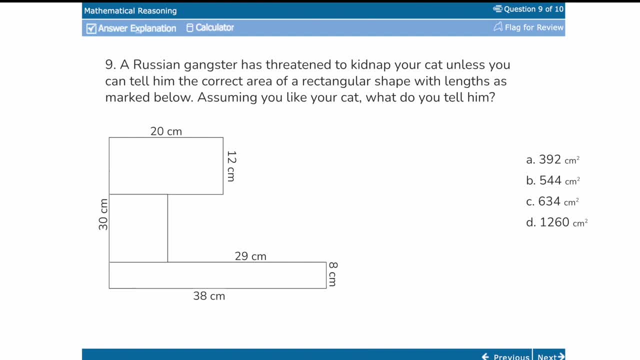 what the area is going to be. but if I draw in some lines, now I have three rectangles. I can deal with a rectangle. Let's do it. The first rectangle: 20 times 12, easy, right, know, basically easy. um 240, great, this one we don't know, we don't know this side, the whole thing is 30. 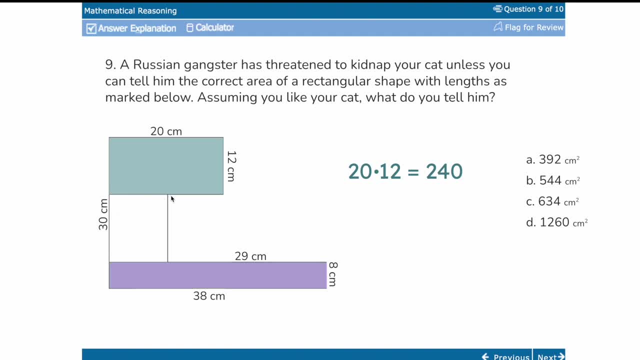 but we don't know this piece of it and we don't know this yet, so let's skip it for now. um, because this is easy, we know 8 and we know 38. that's going to be 304. great, we've done two of the three. 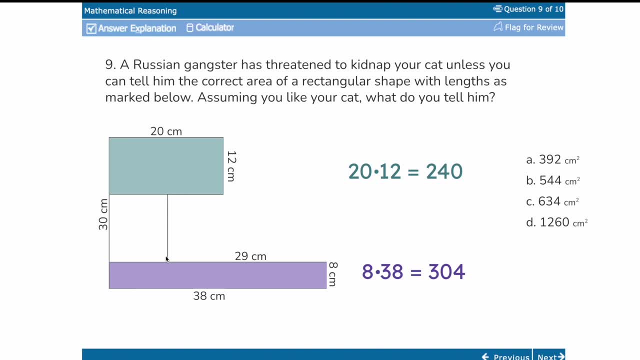 rectangles. we just need to figure out this last piece. well, how do we do that? um, let's look, we know, from the top to the bottom. let's there's just for in the interest of um color completion, let's color it in here. uh, we know, from the top to the bottom is going to be 30. um, well, we know that. 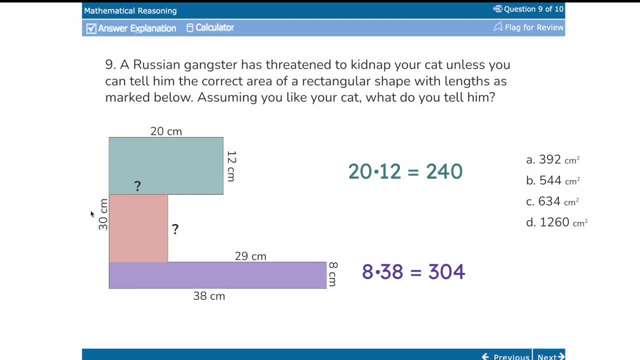 this chunk of it is 12. we know that this chunk of it is 8, 30 minus 12 minus 8. that's going to give us this this side right. um ta-da: 30 minus 12 minus 8- 10. we can write that in. 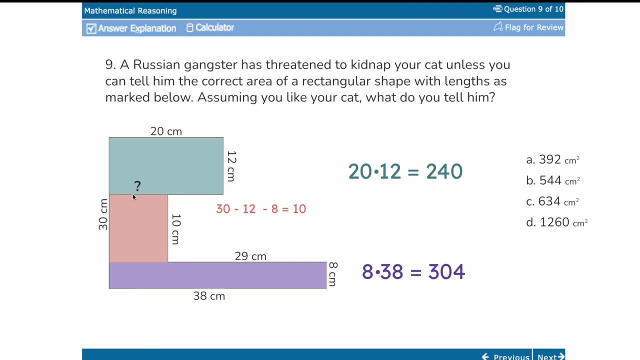 all right, this, this is tricky, this last question mark, because we do know this side, but we don't know this side. so we can't just like take this away, right, but we can use our powers of deduction to realize we might not know this top side, but we do know this bottom side because they're the same. 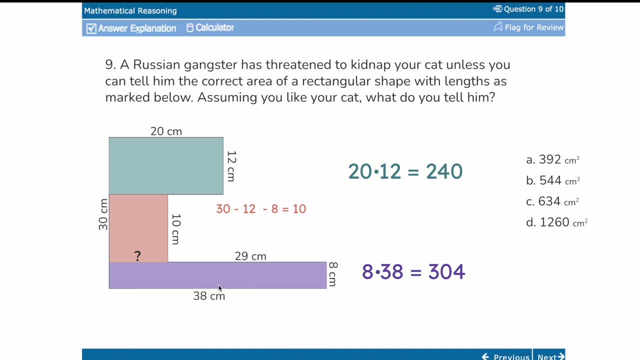 right and we know from this side of the shape to the other side of the shape is 38, but this piece is 29. if we take away 29 from 38, it's going to leave us with whatever this side is. you can think of it also like in reverse, if that, if you're not a subtraction person, you can 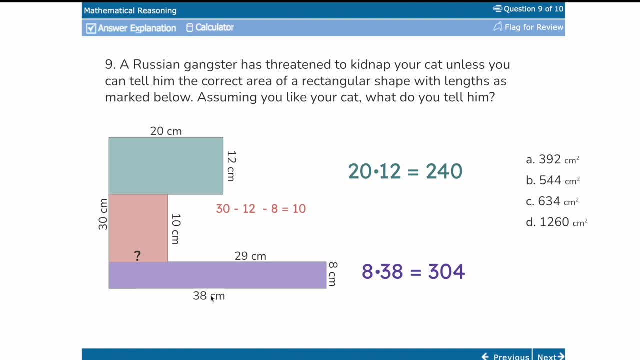 think of it like something plus 29 is going to give you 38. let's figure out that something. all you have to do is take away 29 from 38 and you get 9. great, we've done it. ladies and gentlemen, we have the third rectangle. 9 times 10 is 90. what do you do? it's so hard not to do that stupid chant. 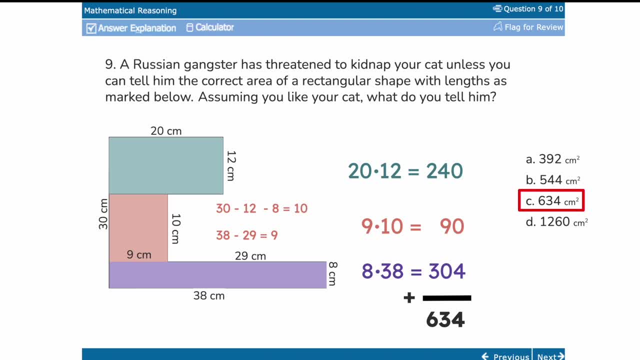 you add them. hooray, there's our answer. okay, that's it. we're going to do it one more time, just for completists out there. we're going to turn this into a perimeter problem. it's the same deal. you have to think the same way. 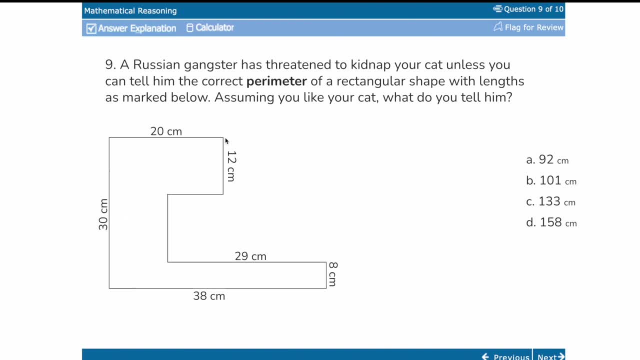 and use the same techniques, but and all the numbers are the same. we just don't know this length. we don't know this length. how do we figure it out? well, you guys remember we figured this out last time. you can go back in the video and see how we did it if you forget it was. 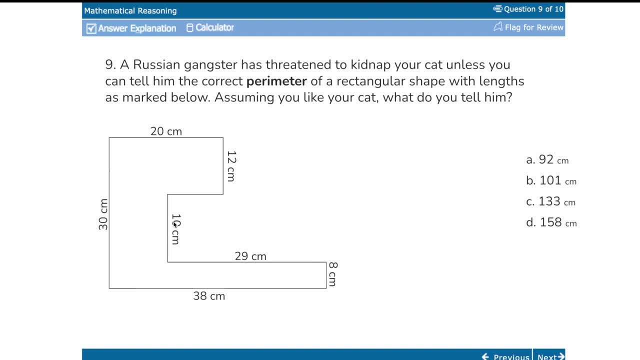 30 minus 12 minus 8 equals 10. what about this, though? um, how do we figure that out? well, we figured this out last time, right, that nine centimeters is this piece, which means nine centimeters is also this piece. and guess what, if we know, from one side of the rectangle to the other side of the 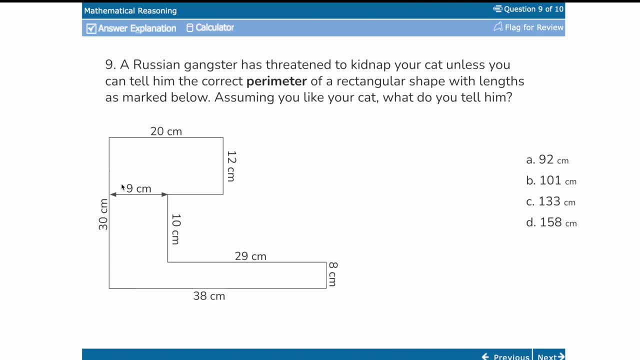 rectangle is 20. you're doing this ahead of me. you're seeing where i'm going, you're learning and doing great. um, we just have to subtract this nine from 20 and that gives up the other side of us, 11.. ta-da, we now know this side is 11 and we know every single side. now, right, we're walking.